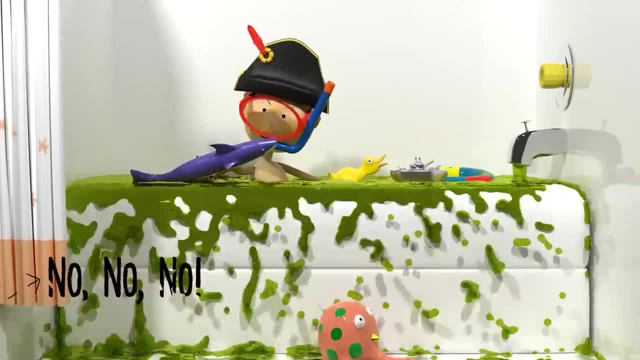 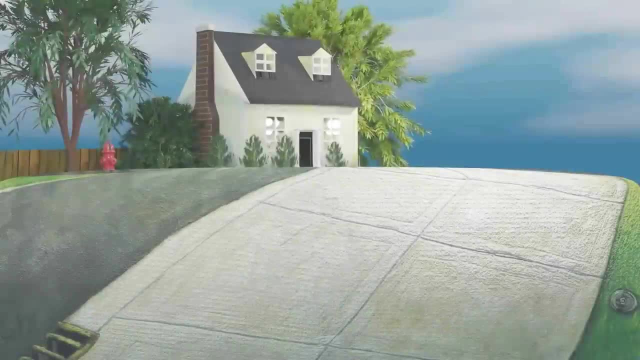 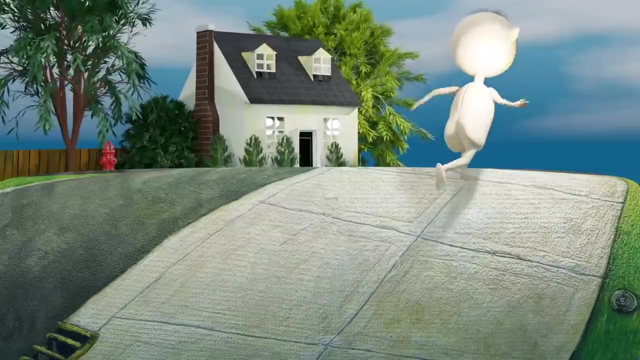 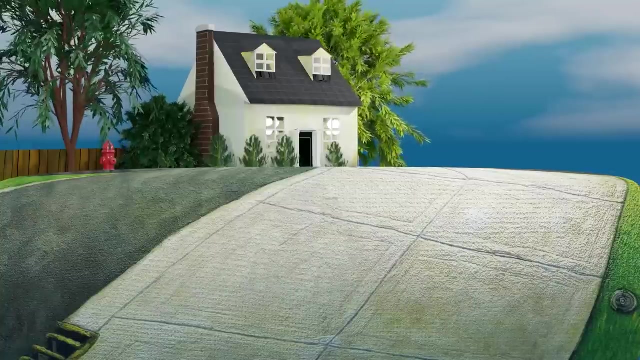 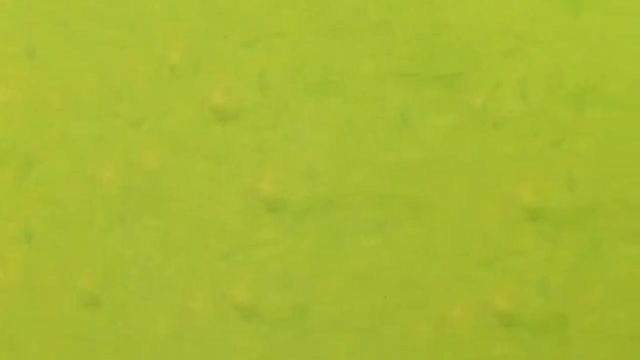 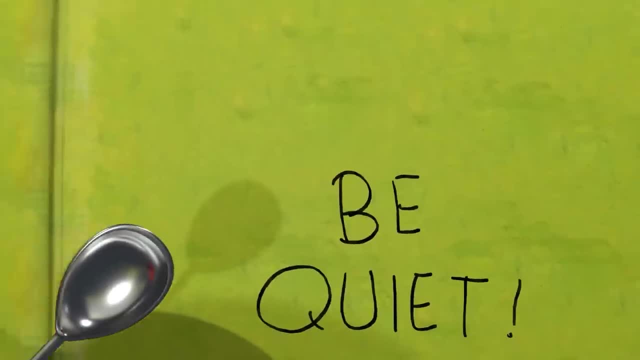 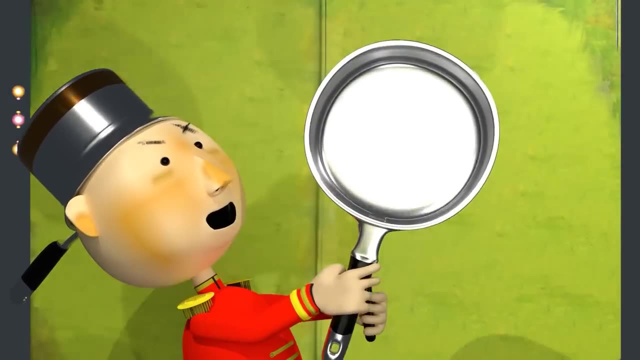 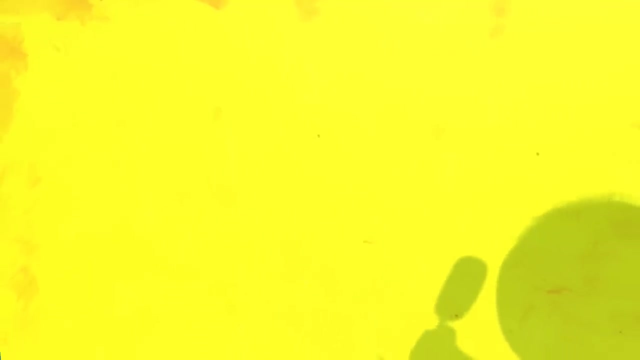 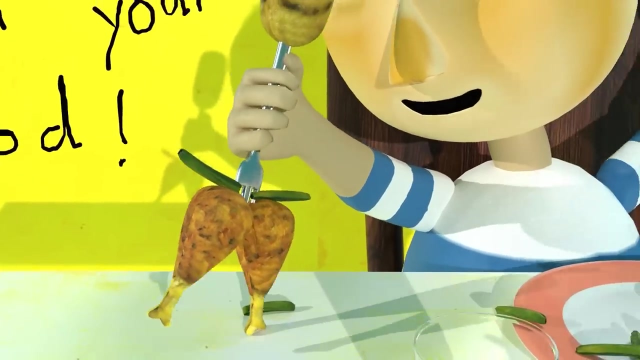 Even when he wanted to eat something, He would play with his food And his mom would say: Don't play with your food And he would not stop playing with his food. If that was my mom, She would go like: Don't play with your food, Ben. 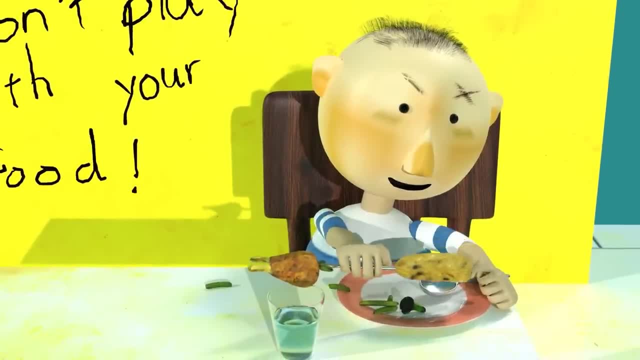 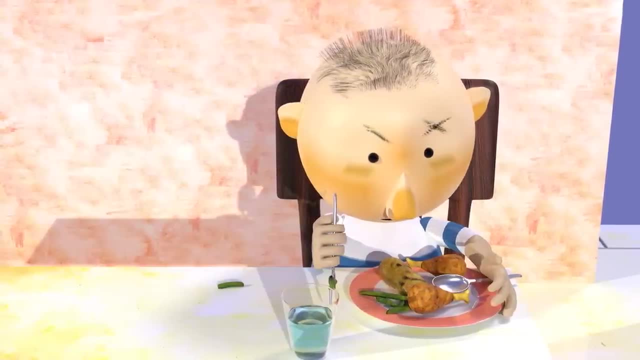 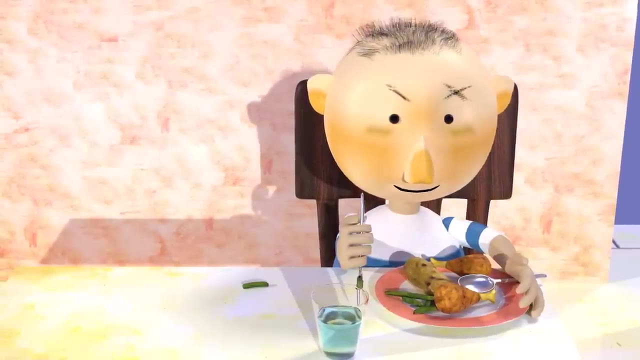 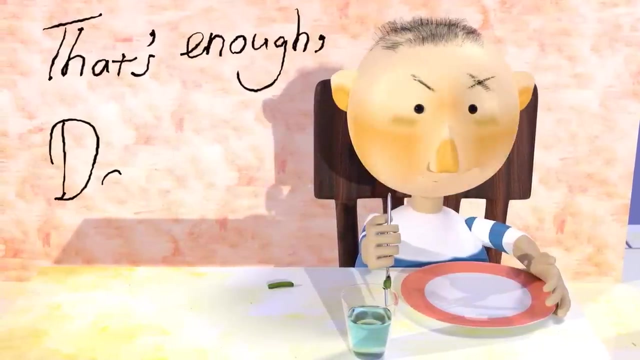 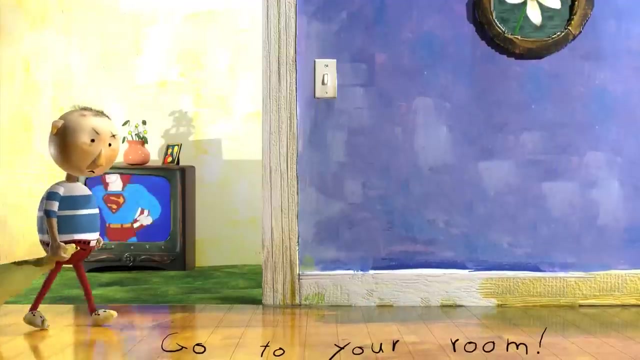 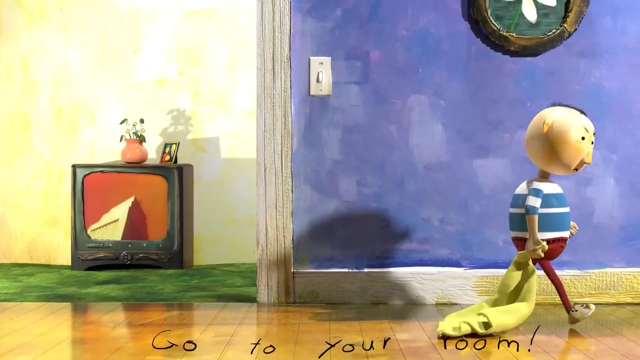 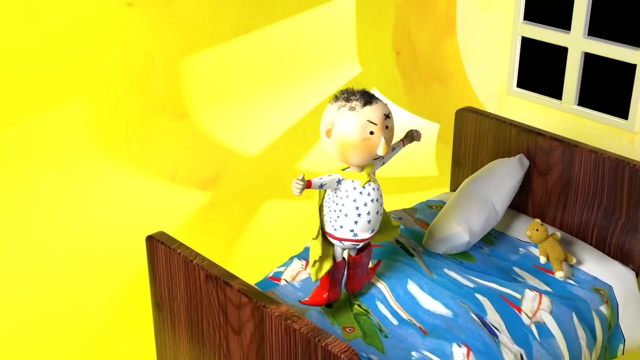 And he would suddenly eat lots of food. Just like that Vanished And his mom would say: That's enough, David, And he would want to stay up late To watch TV. Go to your room. And it didn't end there. He would begin jumping up and down on his bed. 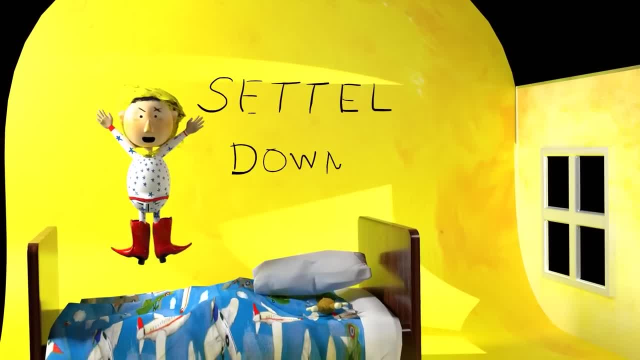 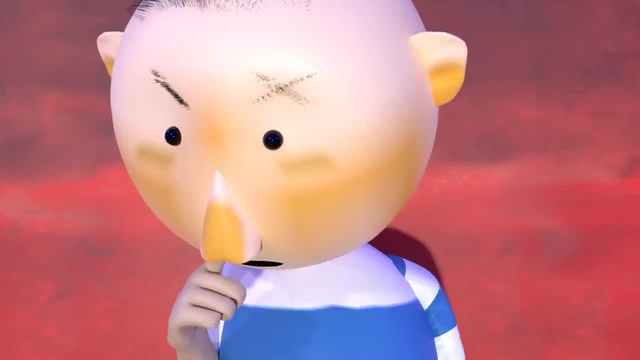 And his mom would say: Settle down And stop moving down all the time And again, Oh Jesus, And again. And also He would love to pick his nose on a daily basis. Mom would often tell him: Stop that this instant.